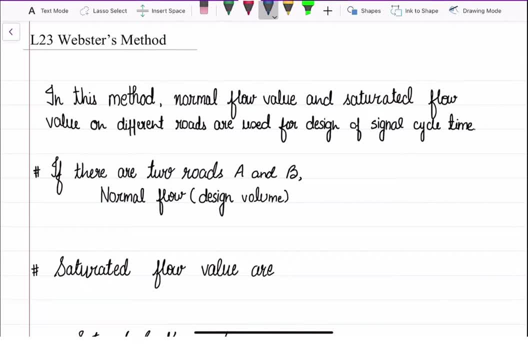 Hello everyone. So, continuing with the discussion on the methods to design the traffic signal timing, the next method that we are going to discuss is the Webster's method. Okay, So before that we had covered the trial cycling method, Then we had done the approximation method And the next method that we are going to do is the Webster's method. All right, So in the trial cycling method we have seen that basically, we assume the traffic signal timing, the signal timing, And then we see, based upon the 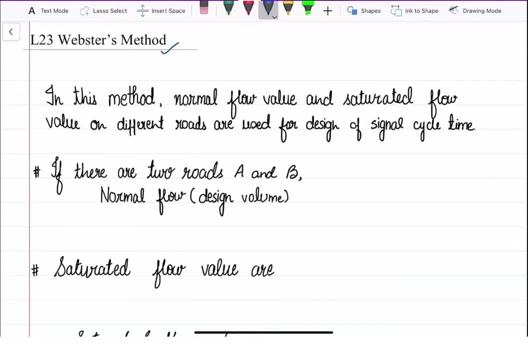 traffic volume if that traffic signal timing is appropriate or not. Right In approximation method we have seen that pedestrians are included and the traffic signal timing is decided taking into consideration the time required by the pedestrian to cross the road as well as the time required by the vehicles to cross the road. 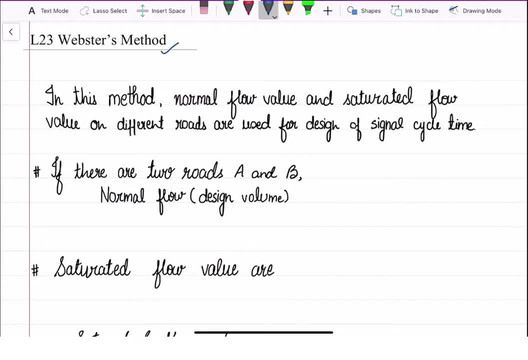 Or cross the intersection. Right Now, in the Webster's method, what we do is we take into consideration the normal flow value and the saturated flow value. Right So we have the intersection, and in that road intersection the road must be having some width, Right So the actual condition, the normal flow value and the 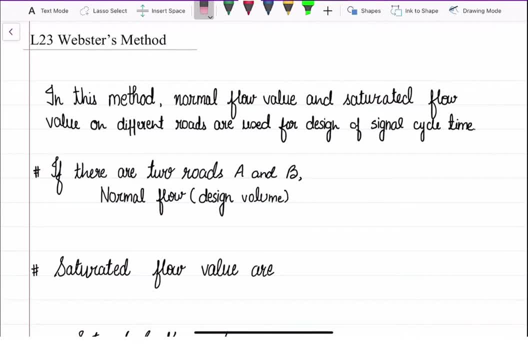 the maximum capacity of the road is considered And based upon that, taking the ratio of that, we find out the total signal time. All right, So this Webster's method: take into account the normal flow value and the saturated flow value of the different roads to design the signal timing. All right, So this normal 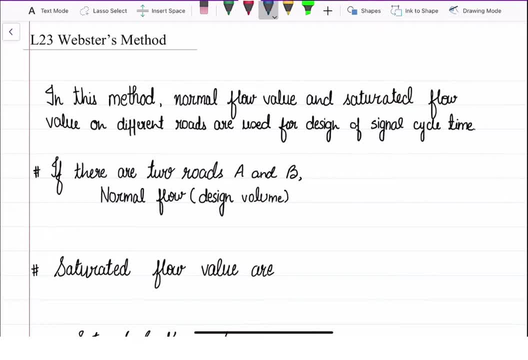 flow value or the running traffic volume or the actual volume of different roads. We will identify them as Q A and Q B, Right? So Q a and Q B is the normal flow value that we have. The saturated flow value is saturated flow value. 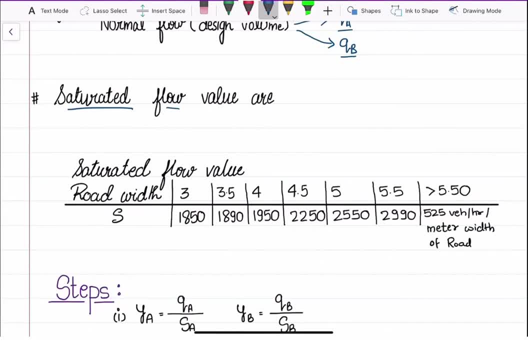 This is, that is level. so, depending upon the width of the road, what could be the saturated traffic flow value for that road is given right. so suppose we have the road as 3 meter, right? if the width of the road is 3 meter, then the saturated traffic flow. 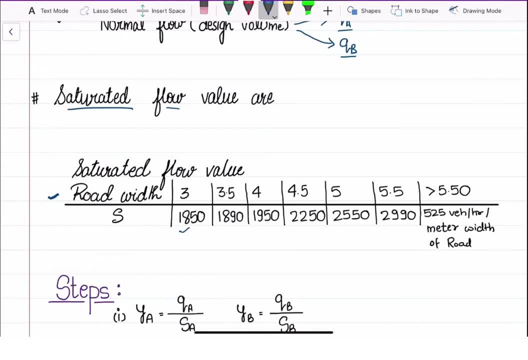 value will be 1850, right, so this goes till 5.5 meter width of the road, and if the available width of the road is greater than 5.5 meter, then we calculate the traffic volume of such roads by taking 525 breakers per hour. 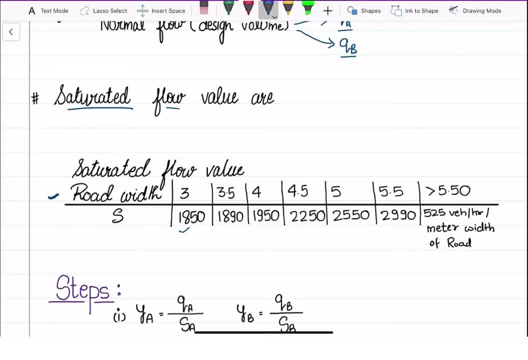 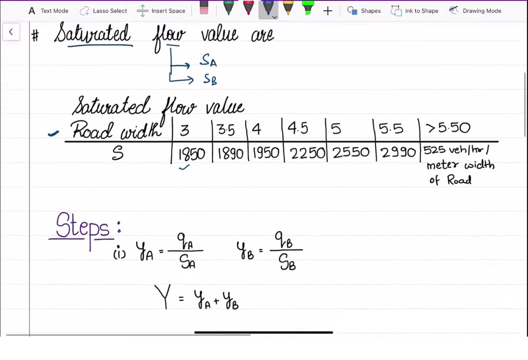 per meter width of the road all right, and through that we find out the total traffic volume, or the total saturated traffic volume of the road. right, so these are saturated traffic flow. we will represent it as SA, SA and SB. right, so moving to the design step. so the first thing that we are, 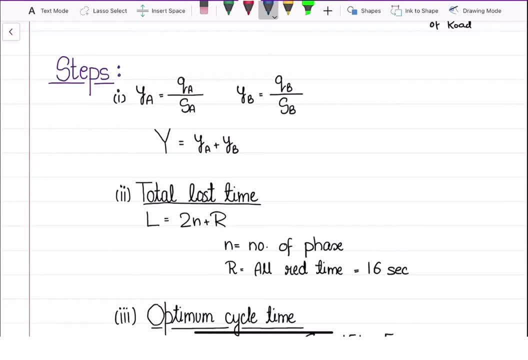 going to do is we are going to find out the ratio of the normal flow value and the saturated traffic flow value right. so your YA and YB- are the ratios of the normal flow value and the saturated flow value right for the respective roads right? and then we will know what the believe is of the sum of each of these florality. such, and then we will have a parameter Y which will be equal to the reach, will be equal to some of your show. we naturally for value and the faktiskt for value. but so we have by a and by B, which is a ratio of normal for value and saturated for value, and we like other why, which is some of M civ Dannendi. a for value. right after this we are gonna find out the total last time, which will be the amount of FA and saying and sustenance value, and we had total value and we are going to find out who lost time, which will be the amount of ruble dancing test, revenue and test no internal stesso value, Navi and Faramti, and that is all article. so if we have an earlier third step, if you proceed to that another slide, you, which would be the ability to move the most well as you, enough to enter in the second computer to show us. 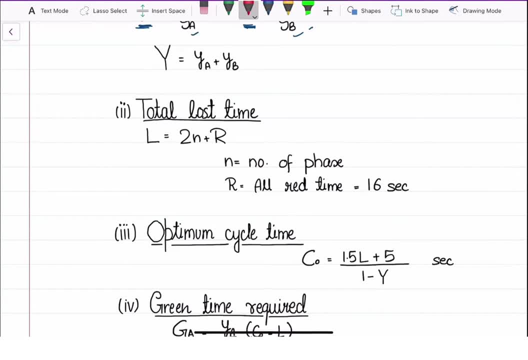 found using the expression: l, equal to 2n plus r. right. n is the number of phase for which we are going to design the signal time. right, and r is the all red time, which, in this case, is taken as 16 seconds, if not specified. right. if not specified, we will take all the time as 16 seconds. right. 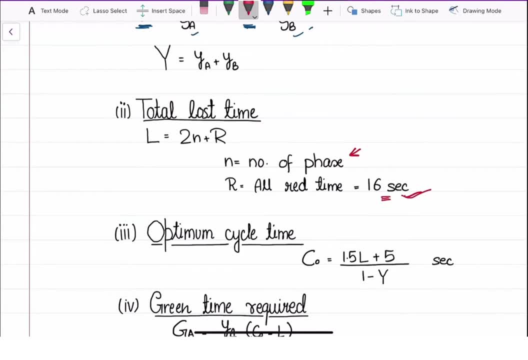 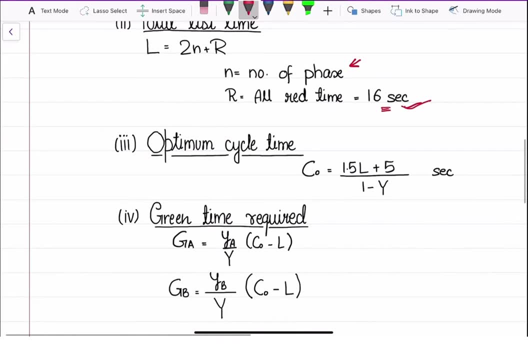 generally for this method, the red time is taken as 16 seconds. okay, and then we find out the optimum cycle time. and optimum cycle time denoted by c naught is found using the formula 1.5 l plus 5 divided by 1 minus capital y. it's a very important formula for your gate as well as other. 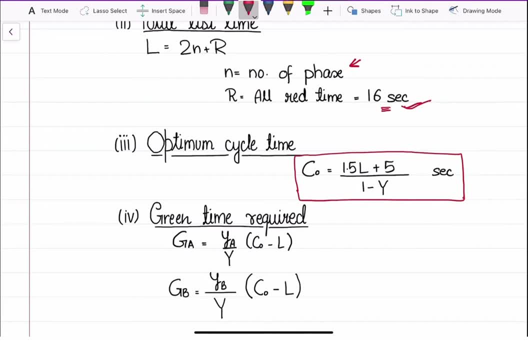 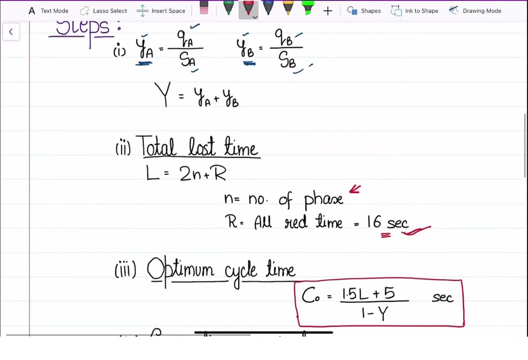 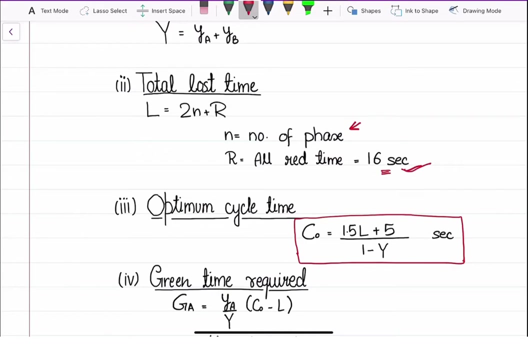 complex examples in objectives, okay, because sometimes directly formula based question comes. okay. so the question may come that you have to design like the normal flow and saturated flow, values are given and the phase is taken as at the two phase or four phase, and then we have to find out the optimum cycle. 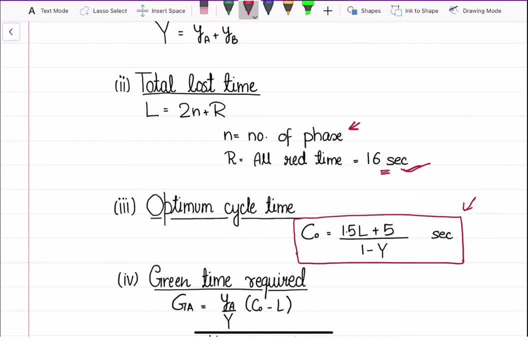 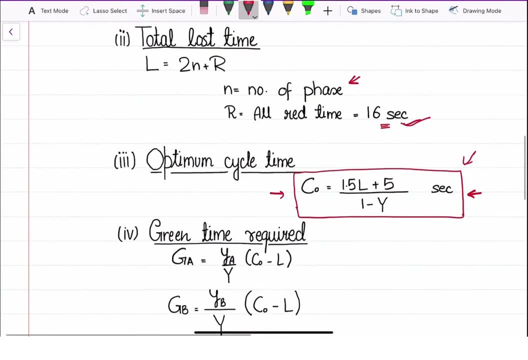 time right. many times it is asked in the gate and in other complex examples which of theATH습니다 did not come every studentuesto very, very long and they go due to the right. so it's a very important formula you should know. okay, now, once you find out the optimum cycle governments based upon the 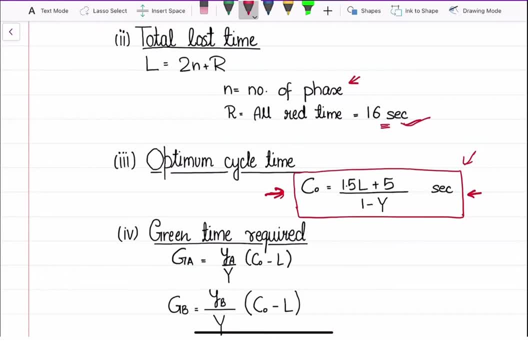 total lost time by the vehicle and taking into account the ratio of the normal traffic flow and saturated traffic flow, we find out the green time required. again, this formula is very important. Why has there been much efficiency in 확 mass event named AC depths? it is not possible to solve because even after the 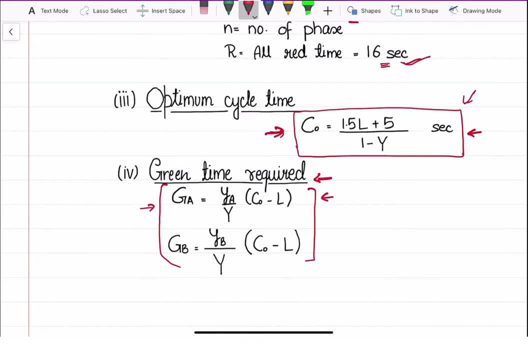 important for gate as well as the computer exams. okay, so your g a and g b are the green times for the respective roads, where the formula for finding out the green time for road a will be y, a by y and bracket c naught minus l right. so z naught is the optimal time that we have found in this. 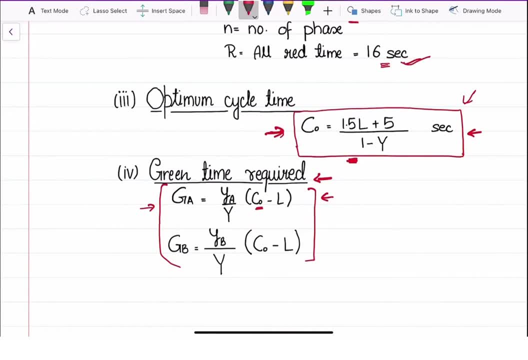 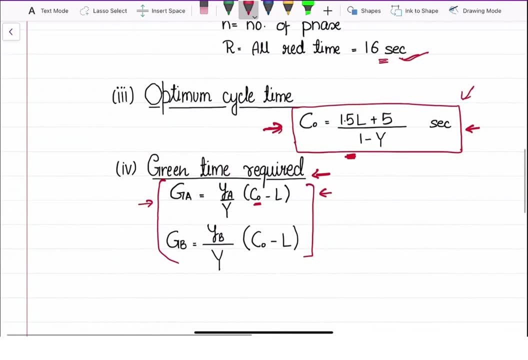 step number three: l is the total loss time that we have found in this step number two, y a by y. we have already found in this step number one, right. so like this, we have to find out the green time required for each of the road. all right, so it's a very short and concise. 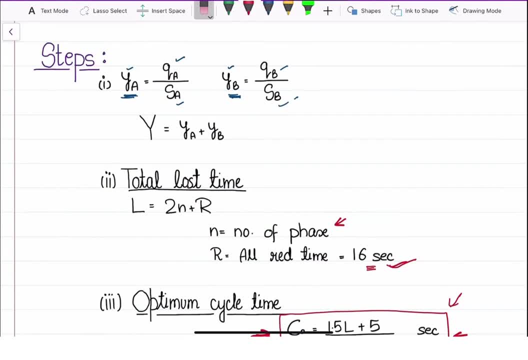 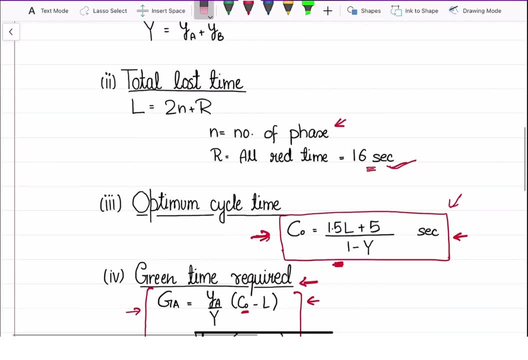 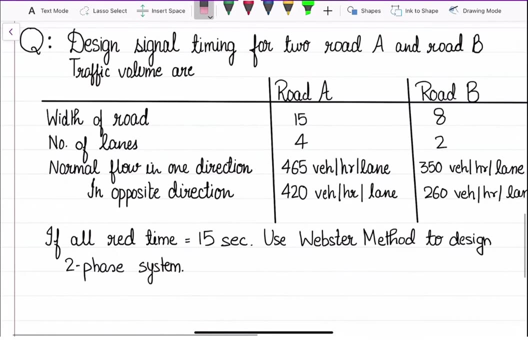 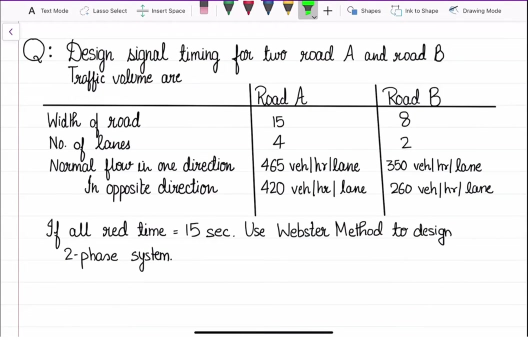 uh method: okay, and is used to design the traffic based upon the normal flow conditions and the saturated traffic flow conditions. okay, so let's do a question to see understand these steps. to design the signal timing using vectors method: right, so we have, uh, two roads, road a and road b. uh, the parameters of the roads are given, right. 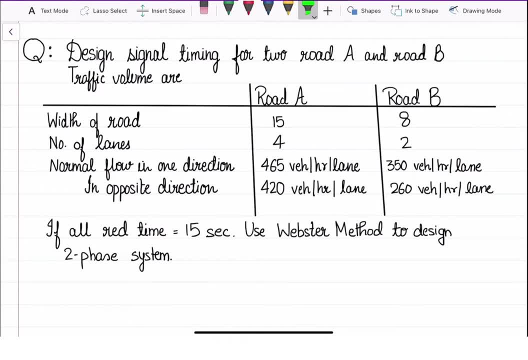 so we have width of the road, uh. for road a the width of the road is 15 meters. all dimensions are in meter right. so width of the road a is 15 and for b is 8 meter and number of uh the normal flow in one direction. 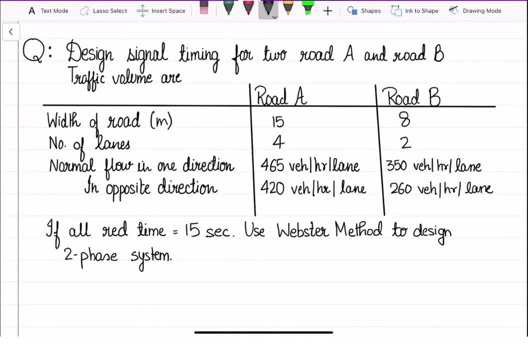 is 465 vehicles per hour per lane and for other is 350 vehicles per hour per lane. on the same road, the vehicles in the opposite direction is 420 vehicles per hour per lane and for road b it is 260 vehicles per hour per lane. right, so here you observe that all that time we have already been 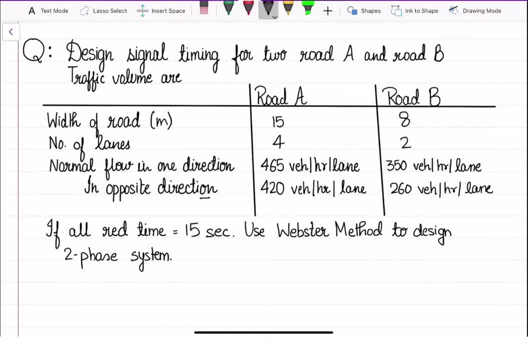 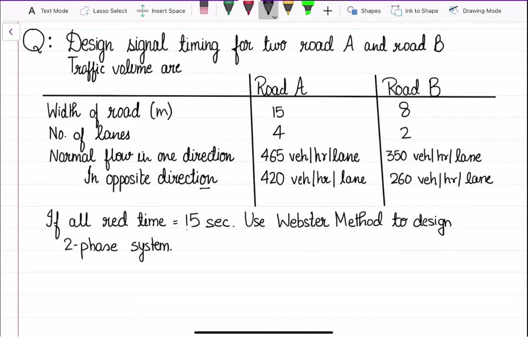 given the number of vehicles per hour per lane, and for road b it is 260 vehicles per hour per lane, and for road 3 and road 2, that is given all that time. that is given fully within your list. then eli just explained why exactly the number of vehicles in the whole road: only 15 🎶. 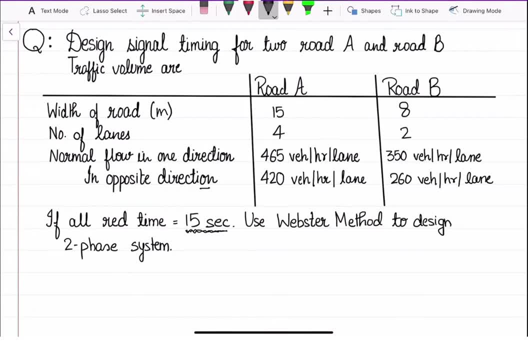 so how we show us the correct KPIs for these world-class vehicles and why we use JSON χ in the world-class vehicles all the time. that is given to us as 15 seconds, right. so if not given, we'll automatically take it as 16 seconds wait, but if it is given, we'll take it as 15 seconds, all right. 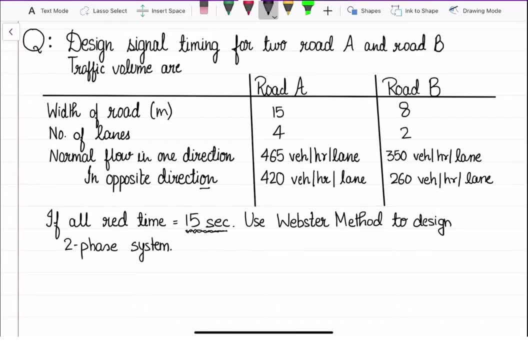 in the web stress method, right. so in that case we basically get the red time. all right. but if we directly suppose in an intersection we move to the we want to design using web stress method, then at that time conventionally the red time is adopted as 16 seconds. okay. 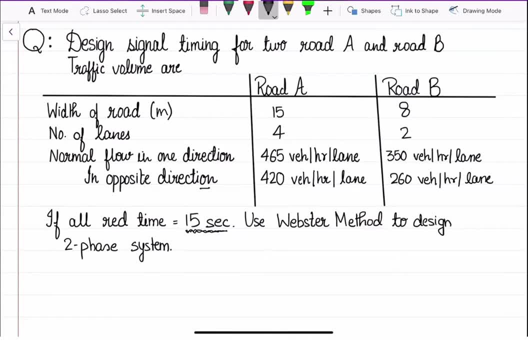 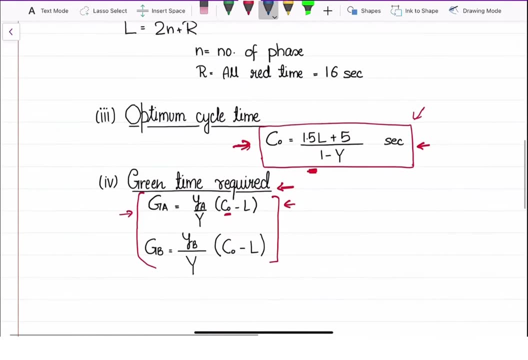 so we use web stress method to design the two-phase traffic signal, all right. so again, i hope you have the pdf open with you all right, in which these steps are written, or you must have noted down but, and you should solve it together, right, then you make it. 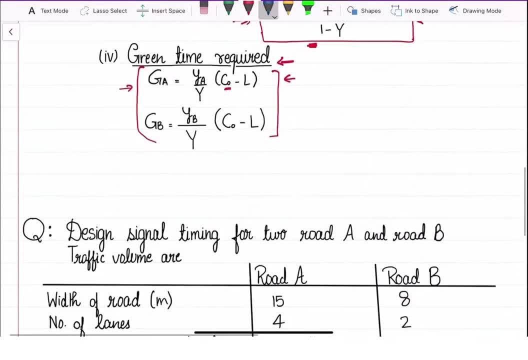 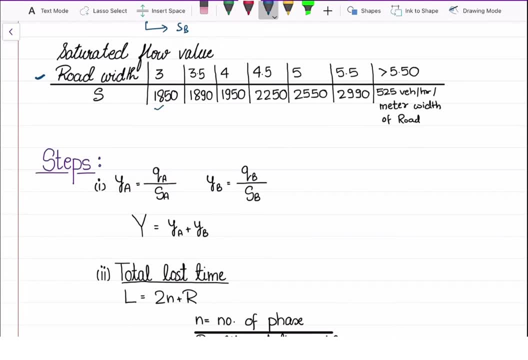 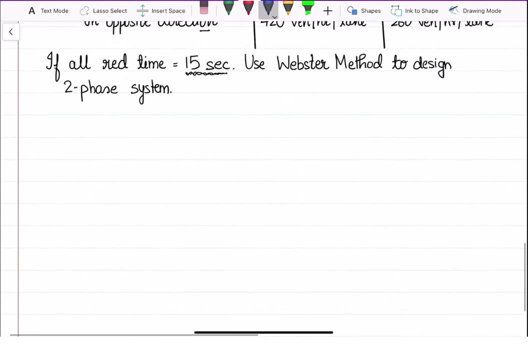 okay. so if we look into the first step of the web stress method, the first step is to find out the ratio between the normal flow and the saturated flow, right? so the step one, the step one, is to find out the y a and y b, and from there we have to find out the capital y. 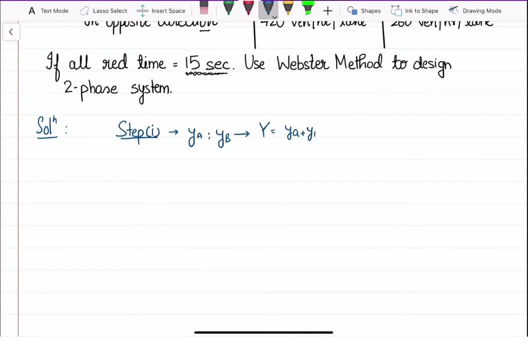 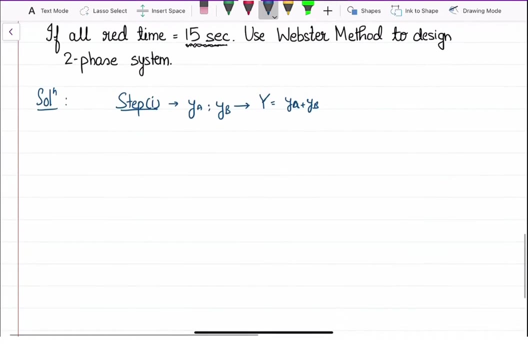 which is equal to the ratio which sum of y a and y b. yes, so y a and y b are the ratio of normal flow to the saturated flow. so for that, the normal flow, let's uh draw the diagram first for the intersection. so from the diagram normally things get much clearer, okay. 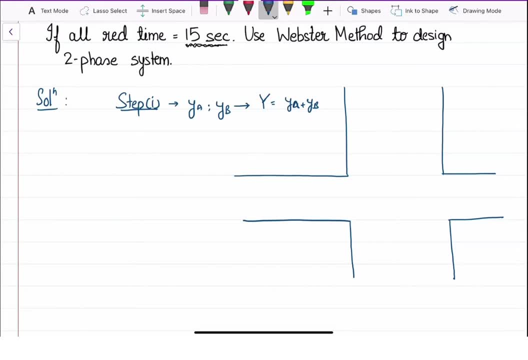 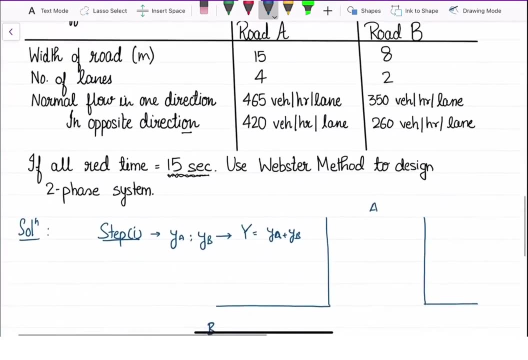 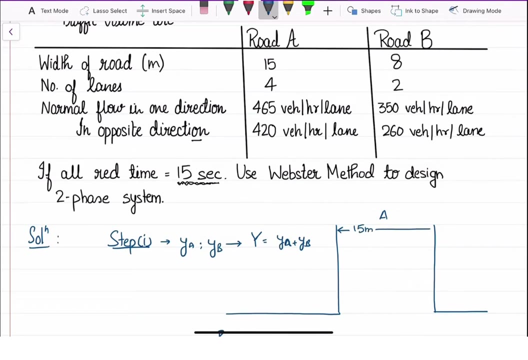 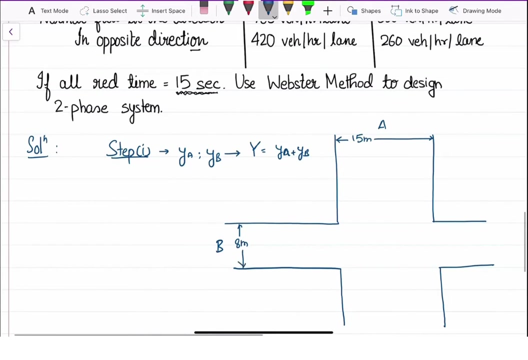 so, uh, we have two roads right. so let's say this is road b and this is road a, right, and the width of the road is a is 15 meter and width of the road b is 8 meter. okay, and number of lanes in road a is four. 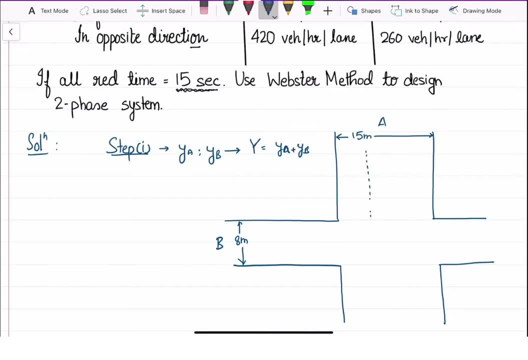 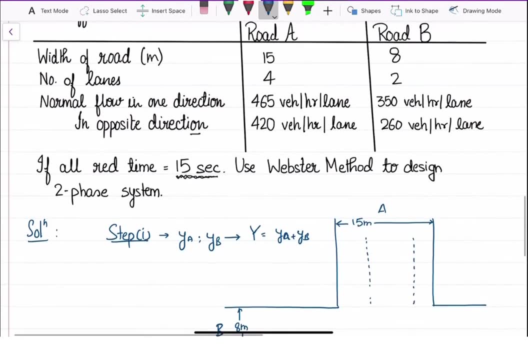 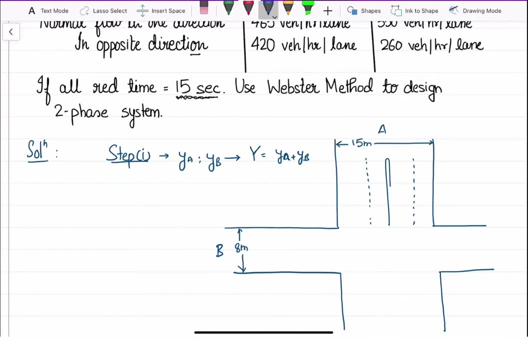 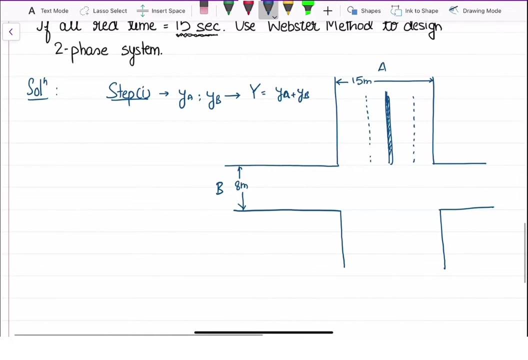 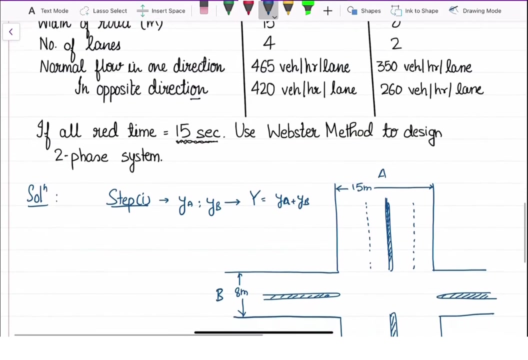 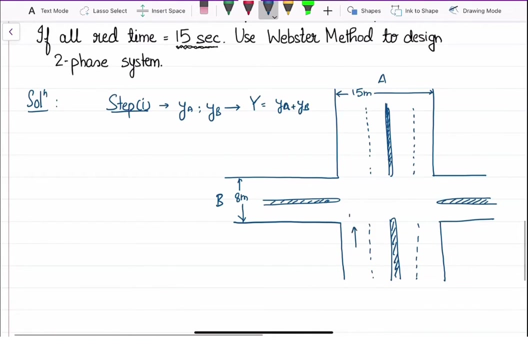 so we have right. and since we have already seen that the vehicles will be coming from uh different, uh opposite direction, so we are going to have the divided in between, all right, then we have to remember that, goed, daily acres. so now that's in terms of the road, a, hence we only have 455 vehicles bending. 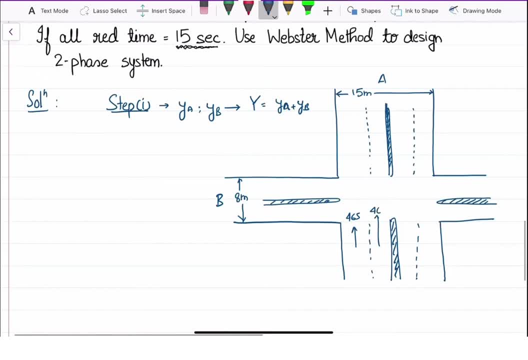 in any full lane than the driveable is 465. so since we have not even used takeout, so you can expect the fastest route germany. 好 well, in first class. lets have a見て see how it works. and in opposite we have 420 vehicles coming from the opposite direction, right. 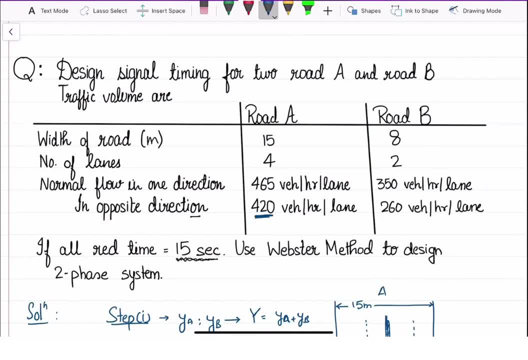 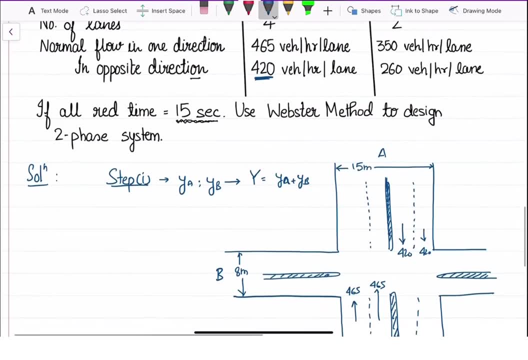 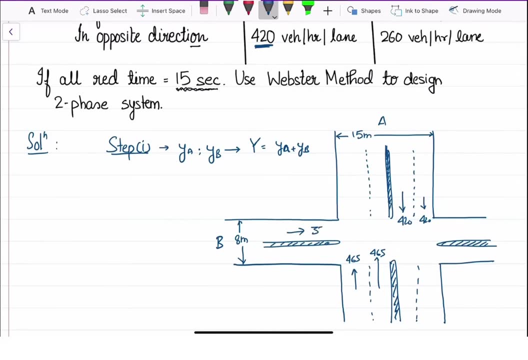 we have 420 vehicles that are coming from the opposite direction. in similar fashion, in road B we have 350 vehicles per hour per lane. right, we have two lanes, so we have from here we have the 350 vehicles per hour per lane and from the opposite direction we have 260 vehicles perhour per lane. ok, 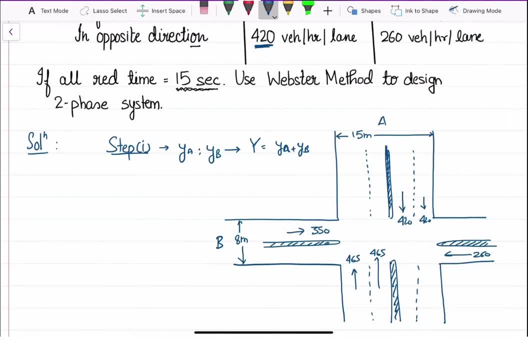 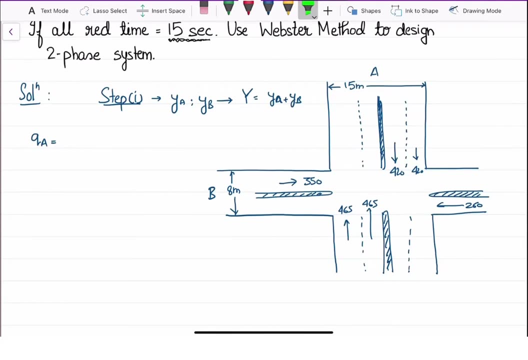 okay, traffic volume taken and vehicles for our lane. so the normal flow that is QA. if you see, just write like we have done, reusable will take maximum value. red, so we have for 35 years are maximum value. so QA is team 465, vehicle per hour per lane. QB: normal flow for the road B highest is 350, right. 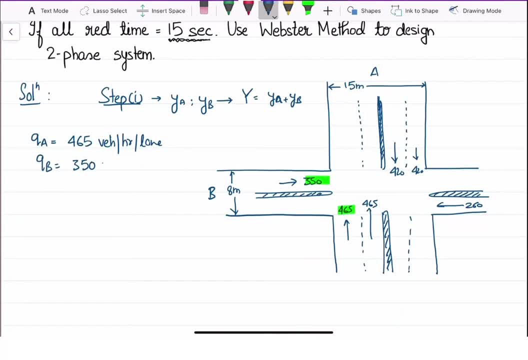 so we will take 350 vehicles per hour per lane. okay, then comes the saturated flow, right, so saturated flow for road A right now. here, the width of the road that we are going to take is 4 meter. right, because this is moving in 4 meter. 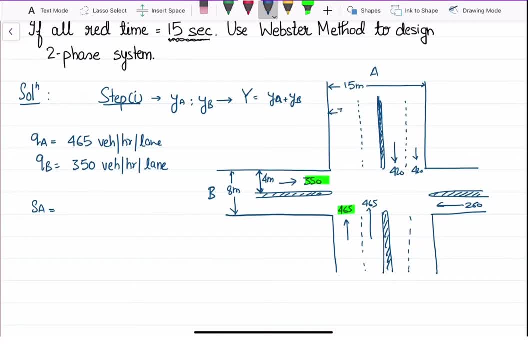 right, and likewise the width of the road that we are going to take is 7.5 meter. for road A, sorry 7.5 meter. 7.5 meter because the vehicles are traveling on 7.5 meters. okay, now for 4 meter, let's put. 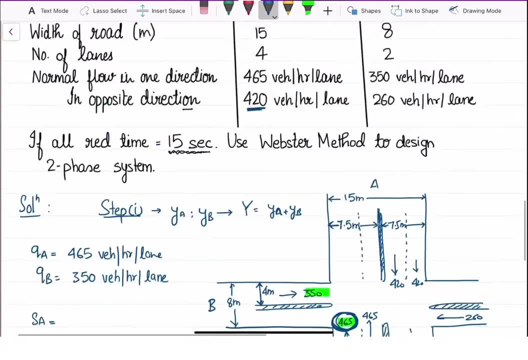 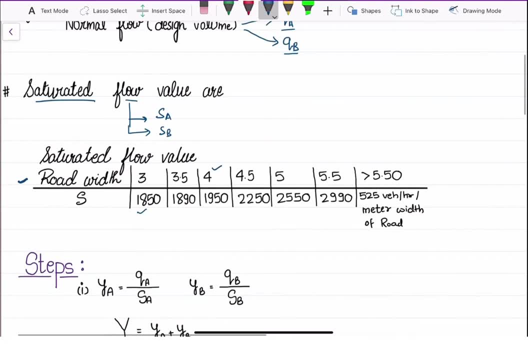 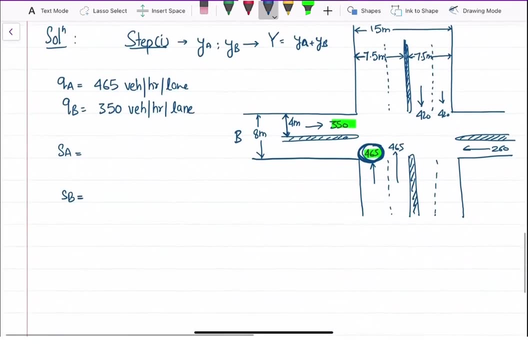 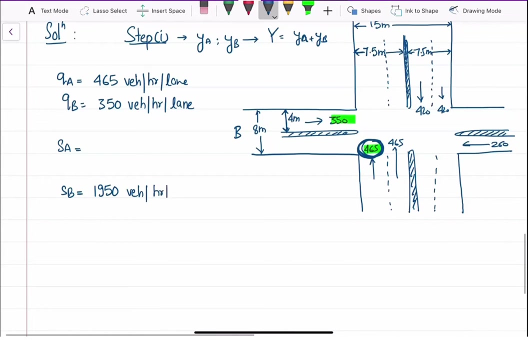 the saturation value for B first. for 4 meter, we have the saturated value table already given to us, right? so here we have the value that is given to us as 1950, right? so we are going to take it as 1950: vehicle per hour per lane. right for A: you see the width of. 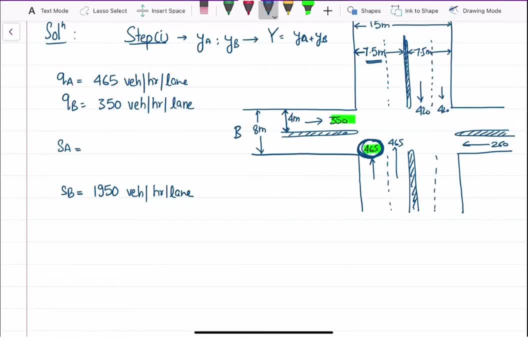 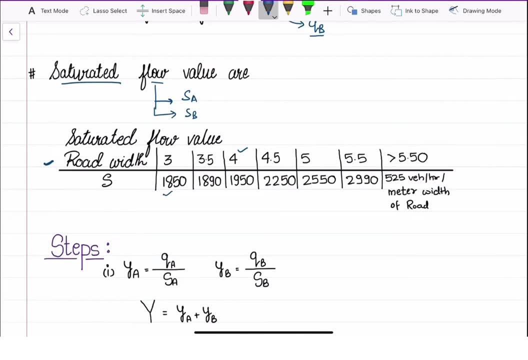 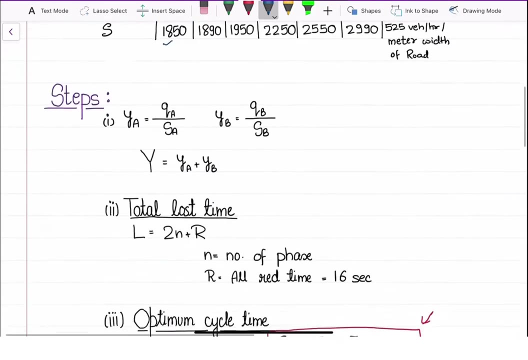 the road is 7.5 meters, all right. so in that case, if the case, if the case, if the width of the road is greater than 5.5, we have 525 vehicles per hour per meter width of the road, right? so here what we are going to do: we are simply going to multiply it with 525. 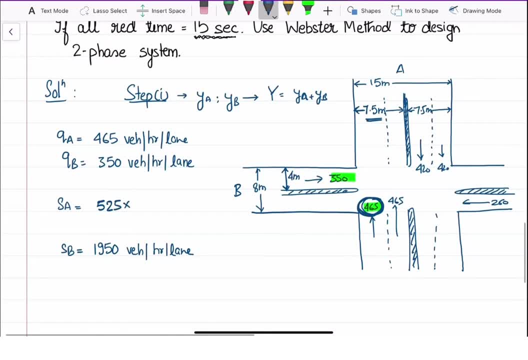 so we are going to multiply 525 into 7.5. all right, so by doing that we are going to have the vehicle as 3.5, 3.5 vehicles. uh, huh, right. so this is the right uh. saturated traffic volume for uh. for the uh. 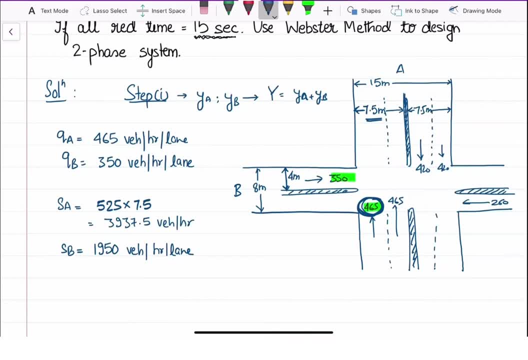 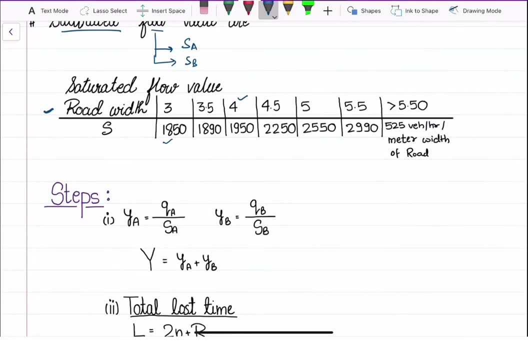 road right, but we take traffic as vehicle per hour per lane, right, very easy, one is selling bill. and this is the list on the physics section of traffic package for So, on audience right, because you see here it is given per meter width of the road, right, so for 7.5 meter width. 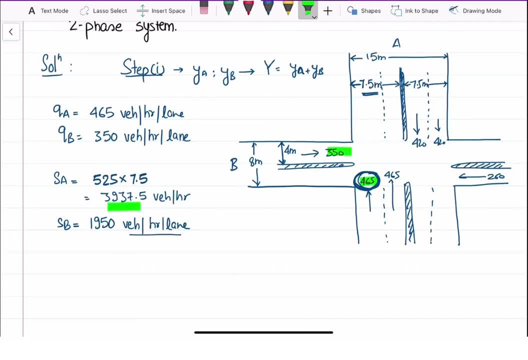 of the road. we have this value right, but we want in vehicles per hour per lane. so here we have two lanes, right, so we have two lanes. so for per lane, what we are going to do, we are going to divide by 2: 3937.5 divided by 2, right? so we will call what is a 1969 vehicle per hour per lane. 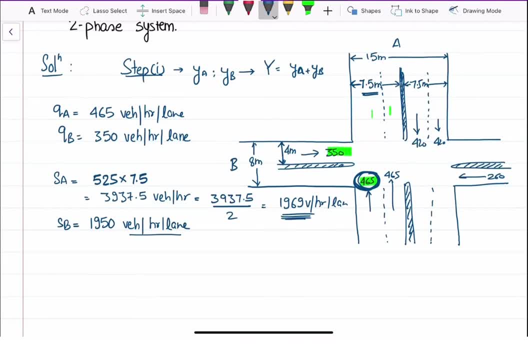 okay, so like this, we are going to have the saturated traffic value per lane for road a. okay, simple, but should be very careful, because when we have the saturated traffic value per lane, we have to be very careful, because when we need to have the saturated traffic value per lane, we need to be very careful, because when we 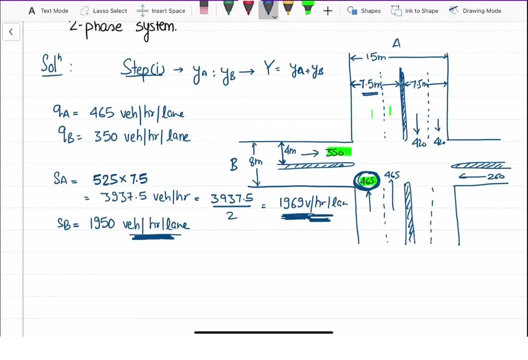 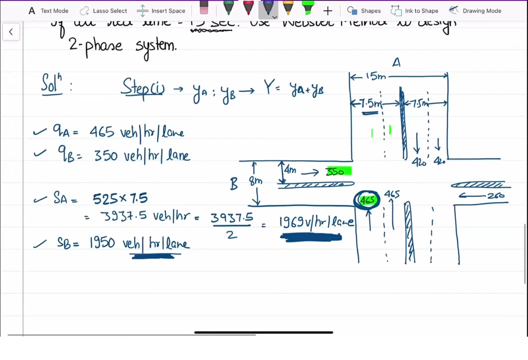 have too many numericals to cover in a very short time period, then this kind of mistakes happens. ok, so be careful about these. right, you have to find out. take up the values as vehicles per hour per day. ok, right, so we have now normal flows and saturated flows, right? 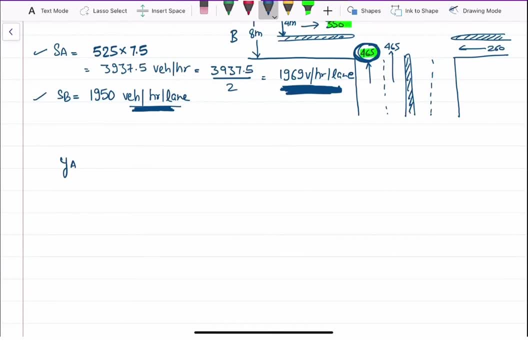 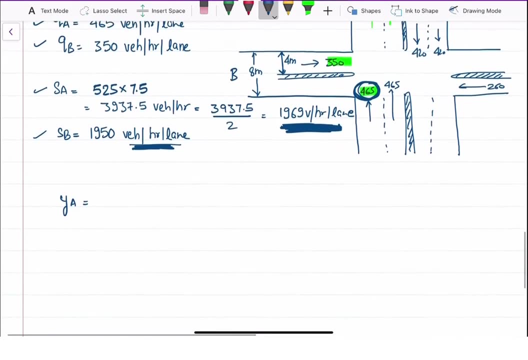 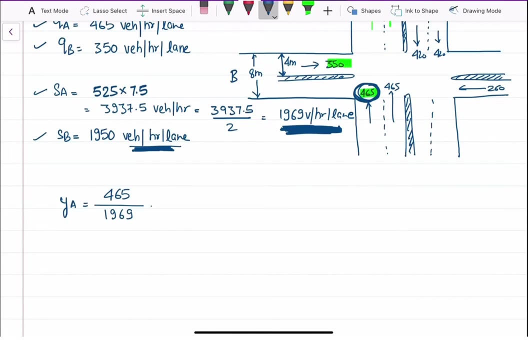 so we can find out the ratio, which is y. y. a is 465 divided by 1969. so it will be 465 divided by 1969. right, so it will be 0.236, okay. and yb. yb is for qb, that is 350, 350 divided by sb saturated flow, that is 1950, that will be 1950, okay, so this. 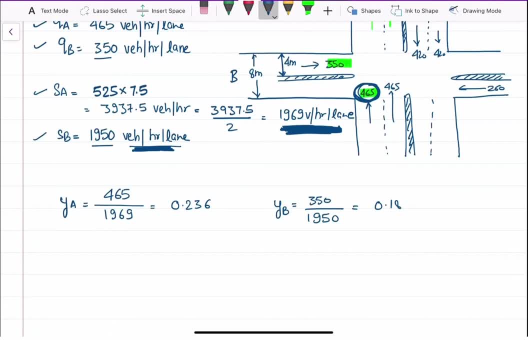 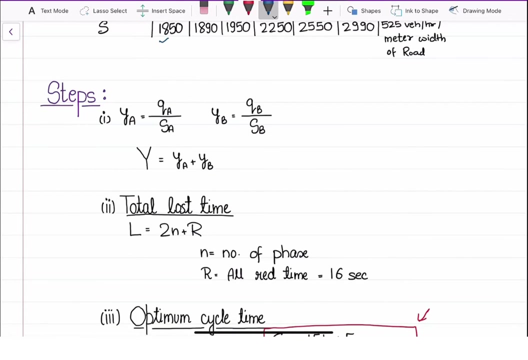 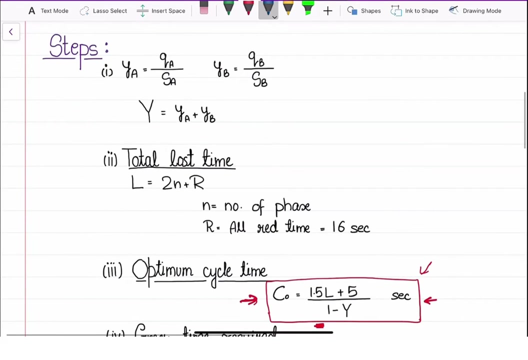 will be 0.18. right, so capital y will be 0.236 plus 0.18, so that will be 0.416. okay, so this completes our step one, you see, instead of one we have: we have to find out the capital y, and we have find out the capital y. now the next step is to find out the total. 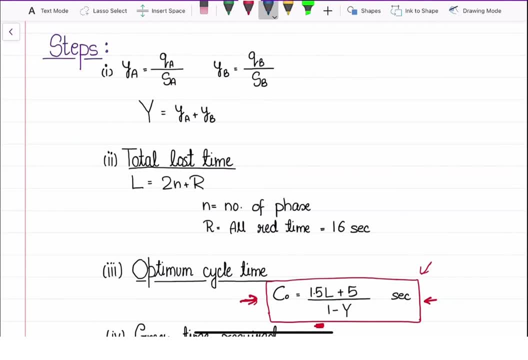 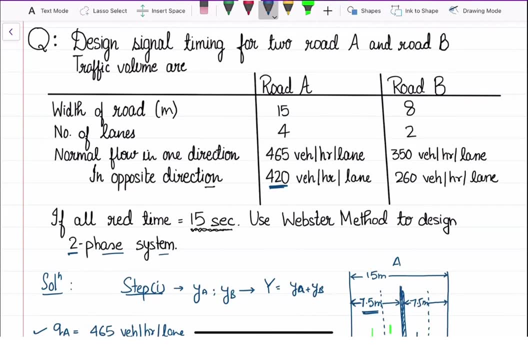 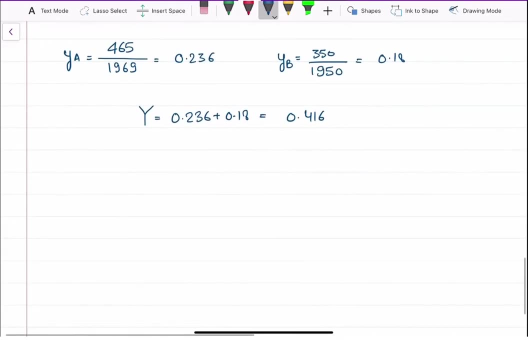 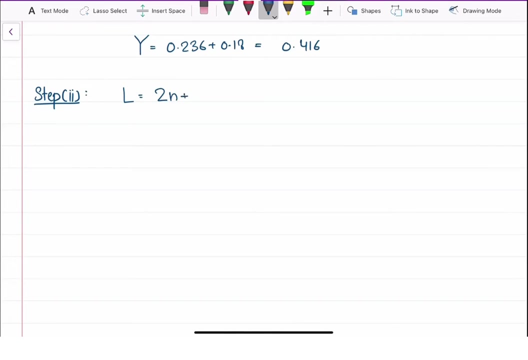 loss time, which is equals to uh 2n plus r. right, so we are designing two-phase system, so here n will be two, the red time we are already given, so we are going to take it as 15, right? so step number two, step two. step two will be to find out the total loss time, which is equals to 2n plus r. okay, so? 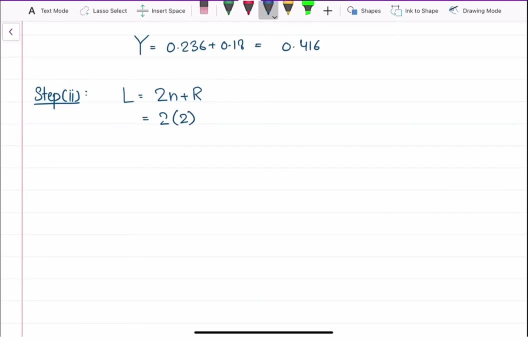 n is the number of faces of signal time, which is 2 in this case, and uh, red light time, we are given 15. so putting the values and we get the total loss time in second. okay, then we have step three, and step three is to find out the optimum cycle. time to find out the optimum cycle. 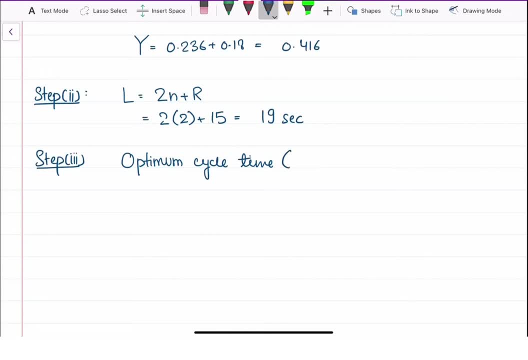 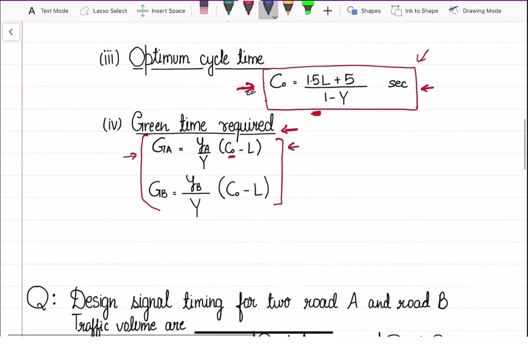 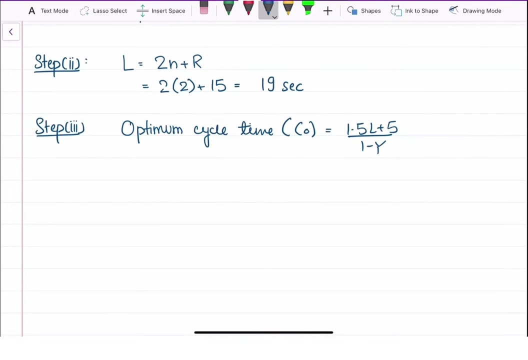 time. okay, so the formula for optimum cycle time is 1.5 l plus 5 divided by 1 minus. all right, let me check. yeah, okay, again, uh, do remember these two formulas. it's very important, okay, so, uh, putting the values so c naught will be equals to 1.5. 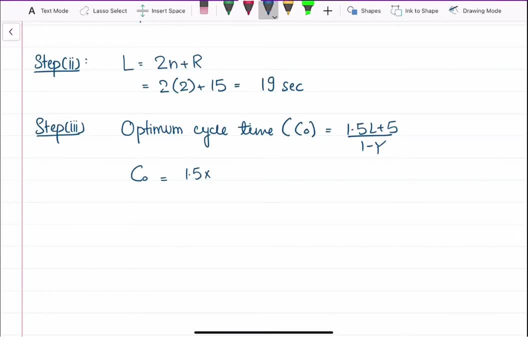 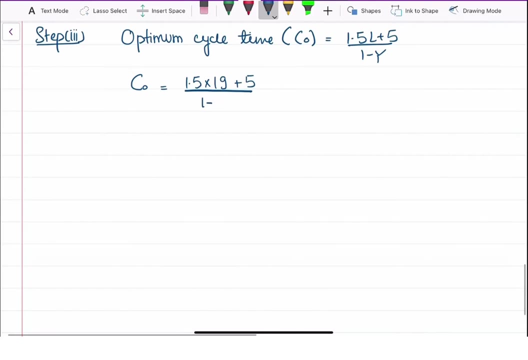 into l. we have already calculated the value of l in step number two, so we are going to put it: l 19 plus 5 divided by 1 minus y, y. we have calculated in step number one, which is 0.416, so it is 0.416, okay. so on solving it, the value will come out as 57.36, which is to 58. 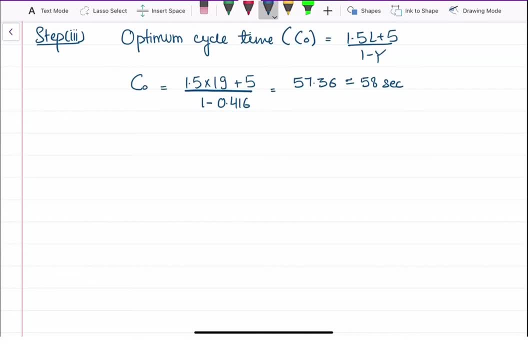 seconds. all right, so we have found out the optimum cycle time: 58 seconds. so now we have to find out the green time. right, we have to find out the green time for the respective roads. so the green time, the green time, green time for Road a will be Y, a by capital, Y into C naught minus L, L. okay. 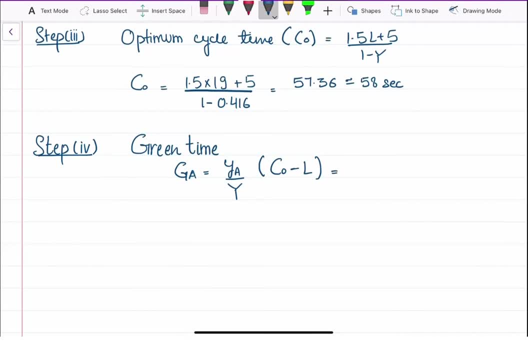 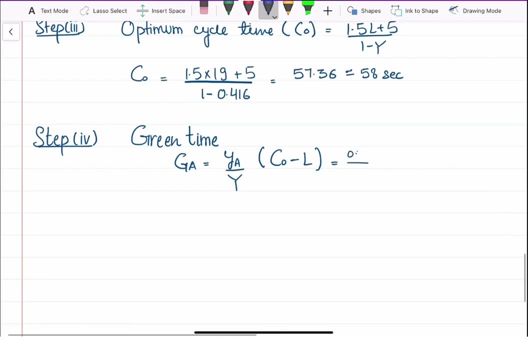 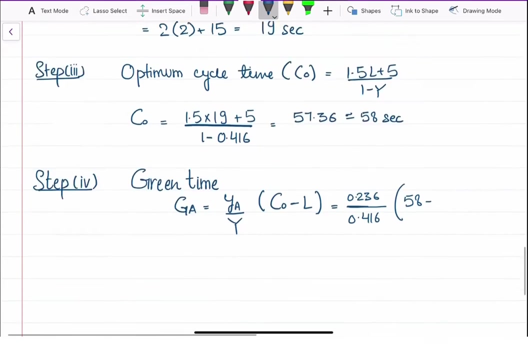 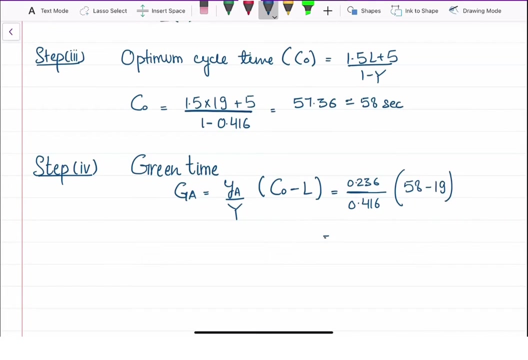 we have already find out the values right. so value of of Why a was open: 2, 3, 6, 0. point 2, 3, 6. value of capital Y was zero. point 5 learned 416 into 58 minus the lost time, which was 19 seconds. okay, on solving it. the. 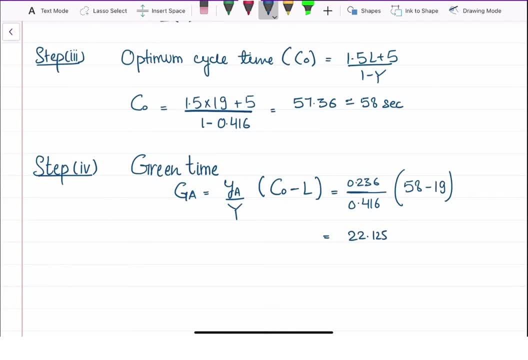 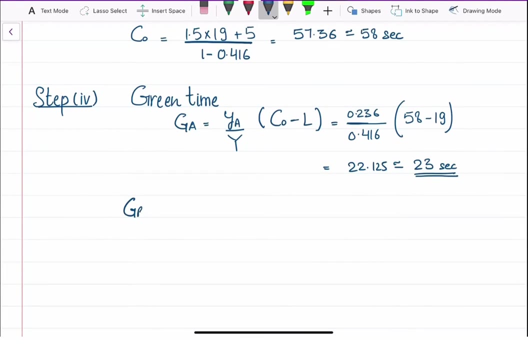 value will come out to be 22.125, which will take as 23 seconds. okay, just solve it as I move along. okay, make sure all the values that I am writing here are correct, but if I'm writing any wrong solution, do let me know. okay, birthday. 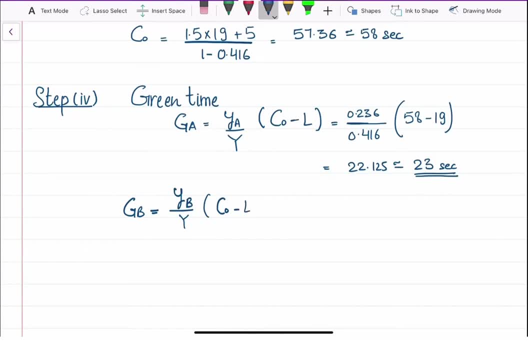 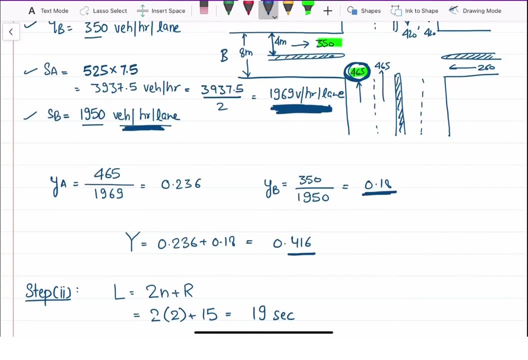 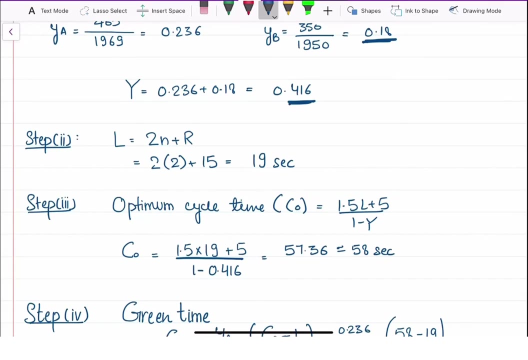 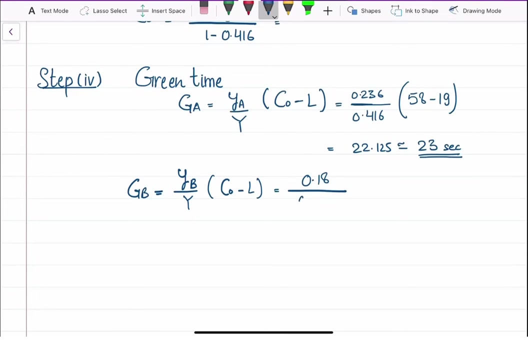 pie Y. C naught minus L. okay, baby, were there, did it. step number one, which is 0 point 1, 8 point. so we will have 0 point 1, 8 Y. we has through, okay, 0.416, and then 58 minus 19, 0.18 0.416. 58 minus 19, okay, so on solving it, the value. 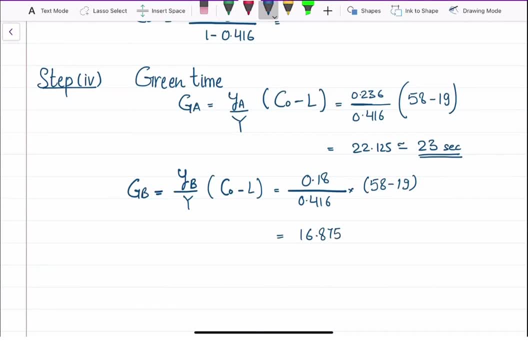 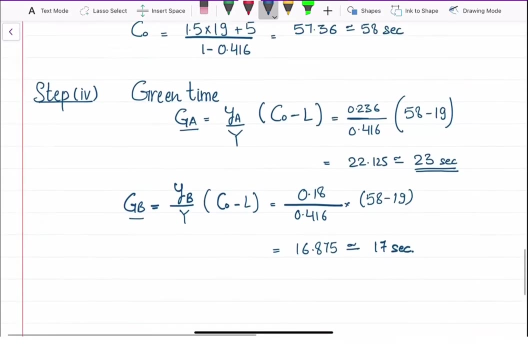 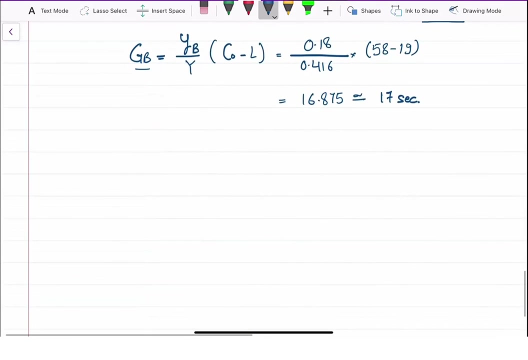 will be 16.875, which will take it as 17 freckles. okay, so now, if you observe, we have the green time, we have the green time for respective roads, we have the ember time will take as 5 seconds, right? so if we want to find out the total, 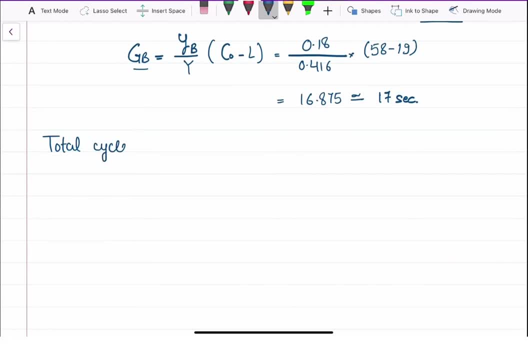 second time the total cycle time. so that will be GA plus AA, GV plus AV. all right, so that will be 23 plus 5 plus 17 plus 5. Oh, the total cycle time will come out to be 50 seconds. okay, so the total cycle time. 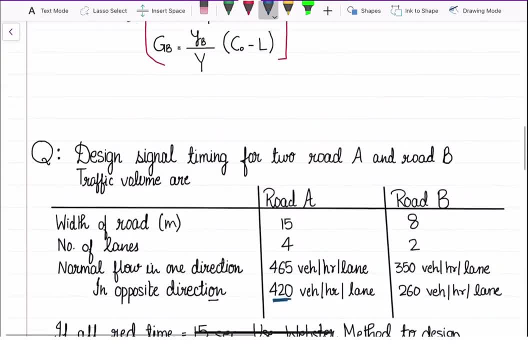 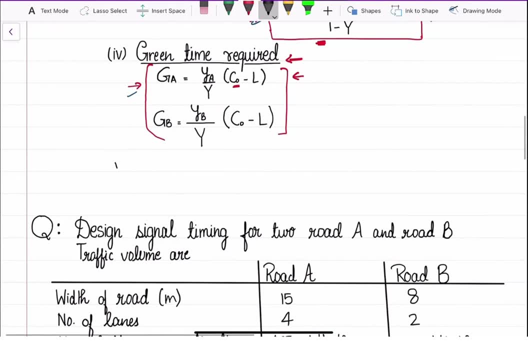 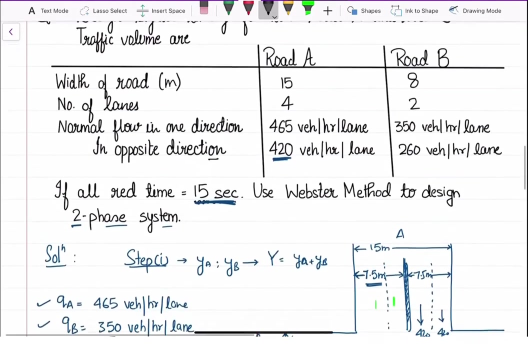 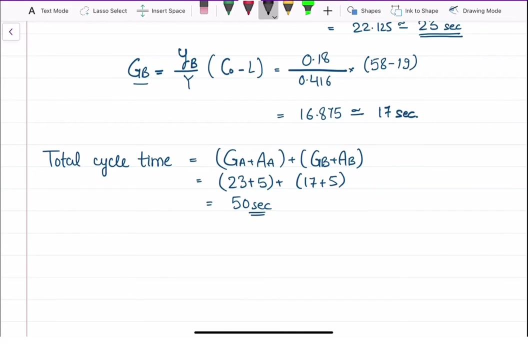 will be 50 seconds. I should write here about the total cycle time. the total cycle time will be equal to GA plus AA, GV plus AB. okay, so like this, basically, we solve the, the, or we find out the traffic traffic cycle time using the Webster's method. all right, so this is how. 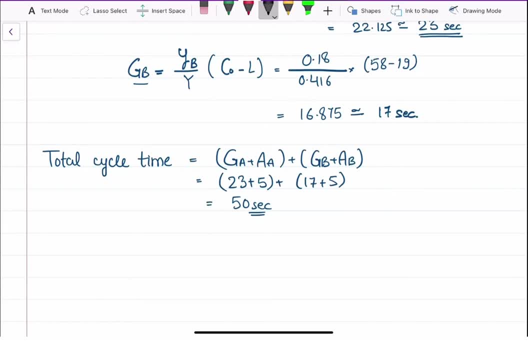 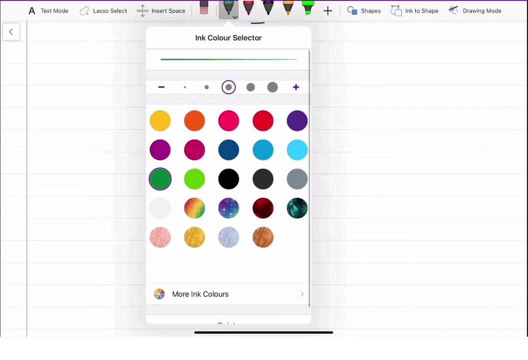 it is done. okay now. so the last method that we have is the IRC method. okay, now, in IRC method nothing unique is in IRC method. what happens is it's a combination of approximation method and Webster's method. okay, so I'll just cover here only we have 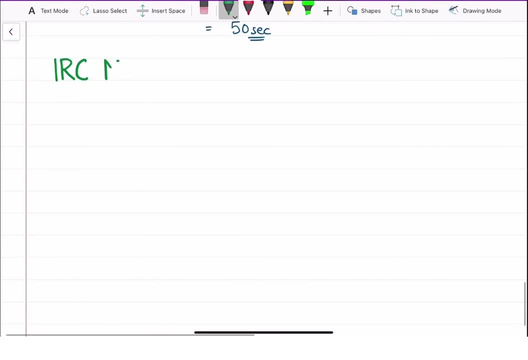 IRC method. it is the kind of method you use in ORC, The, So in Ossetian method is worth using. GV就是 the number of will take up to 12x. will take up to 158 method. that is, this is the fourth method, right? so IRC method is a combination of this method. 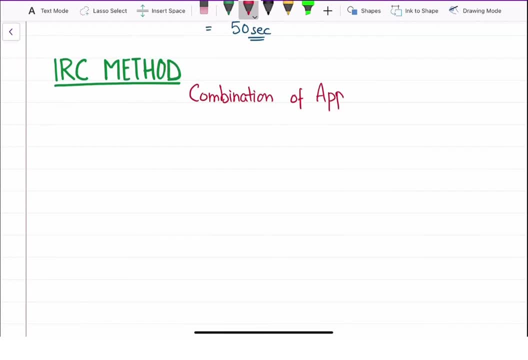 is a combination of approximation method, combination of approximation method and Webster's method. okay, is a combination of approximation method and Webster's method. so basically what we do is we design the design, the traffic signal. we design traffic signal using approximation method. okay, and then what we do? we check the. 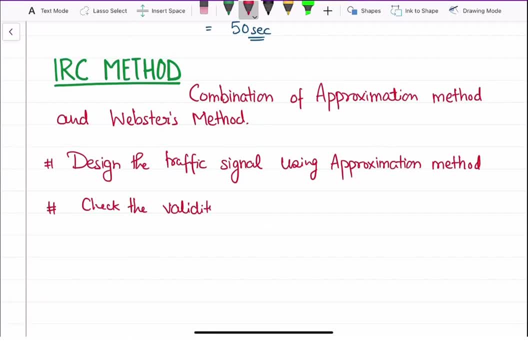 the validity. we check the validity. validity means the minimum green time, minimum green time using Webster's method, minimum green time and the cycle time also okay in green time and minimum cycle time using webster's method okay. so simply put: first we solved by approximation method and